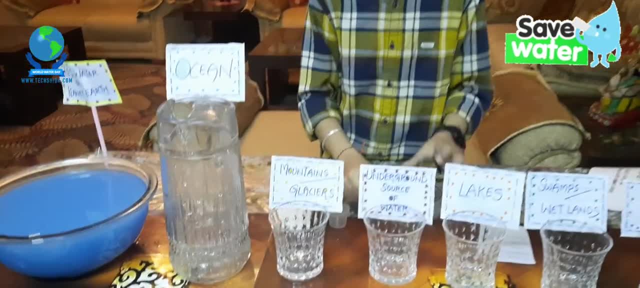 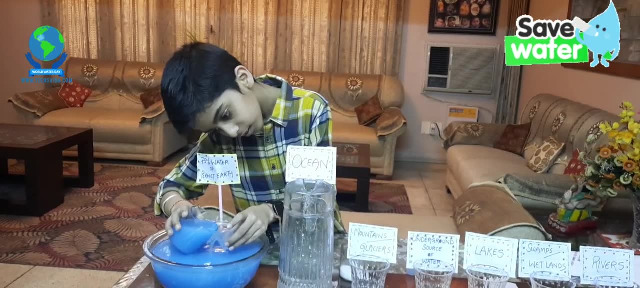 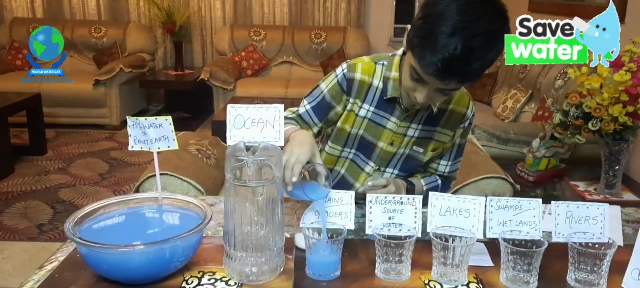 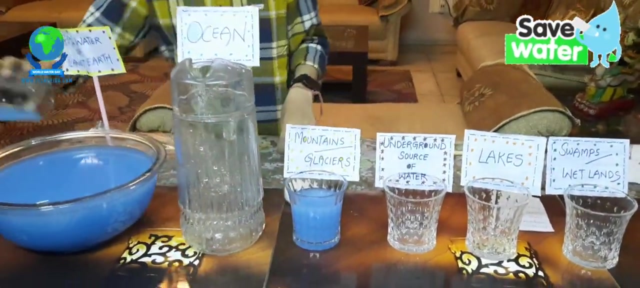 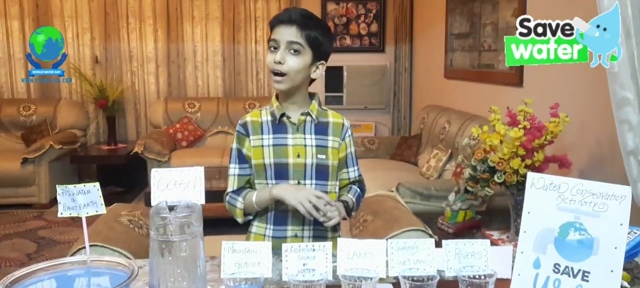 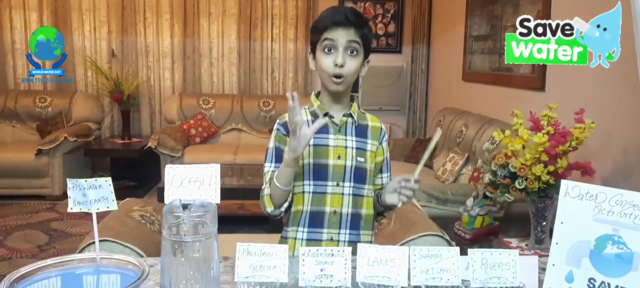 water body, mountain and glaciers. so you can see, this water is in category of mountain and glaciers. so now let's turn off underground sources of water. and do you know how much water underground and sources of water have? 9 ml, only 9 ml out of 1000 ml. so now i am going. 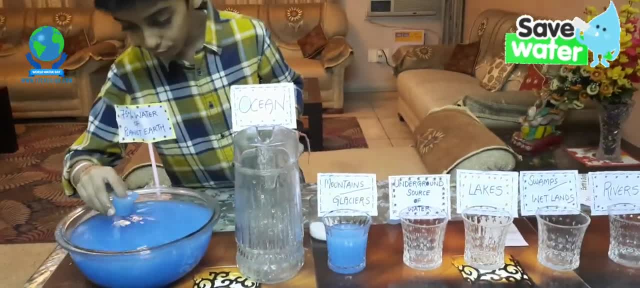 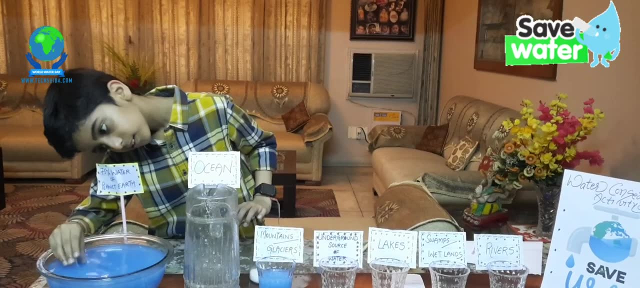 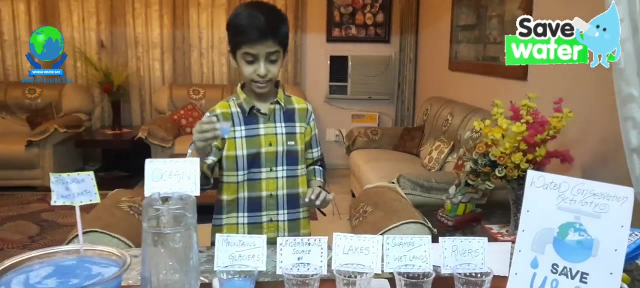 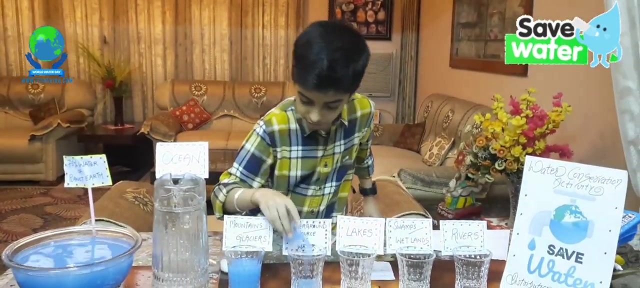 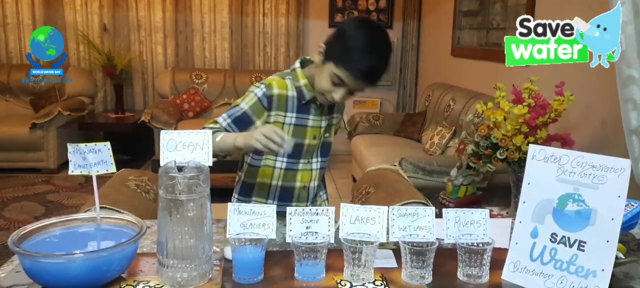 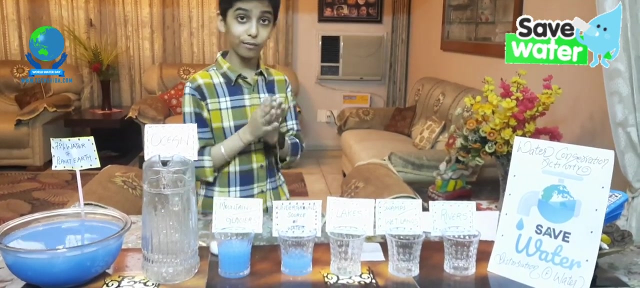 to put 9 ml of water into the category underground sources of water. a little bit more, and this is 9 ml. one more, and then 9 ml is completed. so this is 9 ml. now let's turn off lakes, and do you know how much water lakes have? 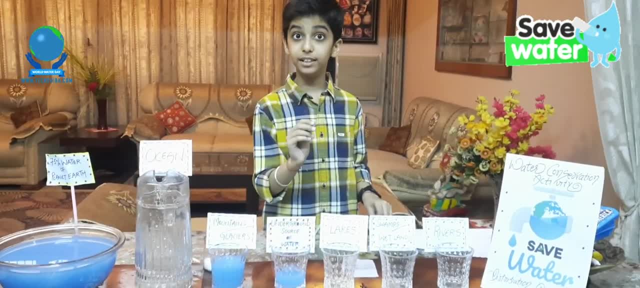 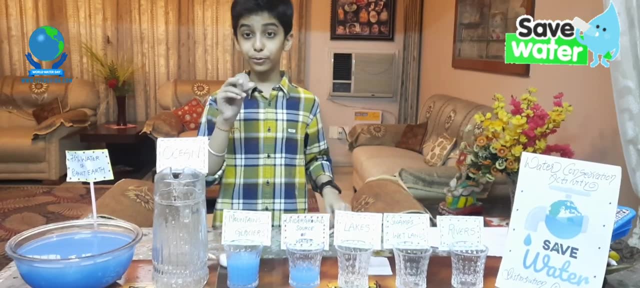 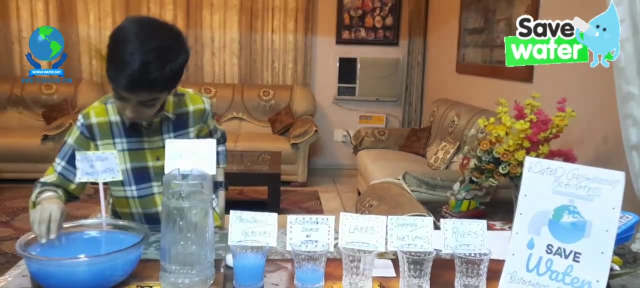 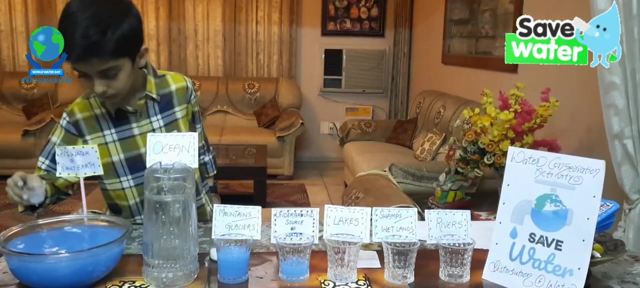 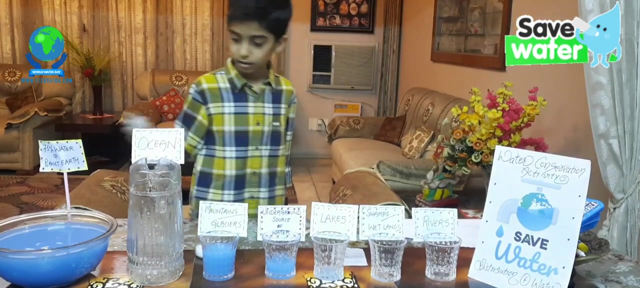 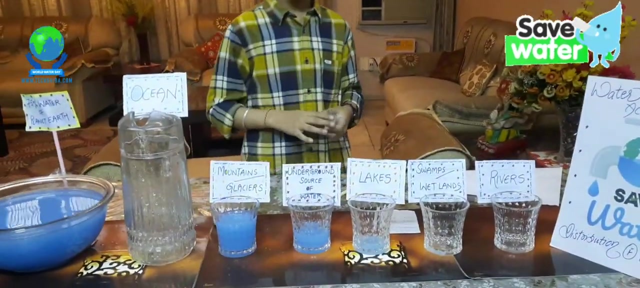 only 0 ml. 0.08 amount of water in lakes: 0.08 ml. can you imagine? now I'm going to put 0.08 ml of water into the category lakes, a little bit more and one more and done. this is the category of lakes. now it's turn of swamps and wetlands. and can you get? 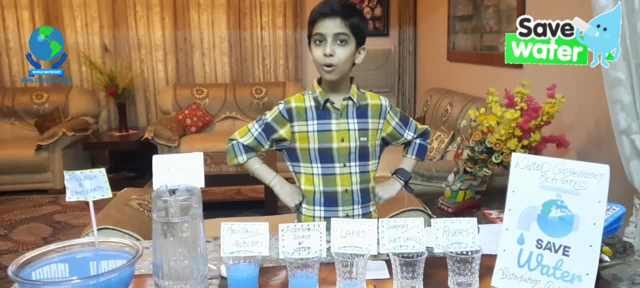 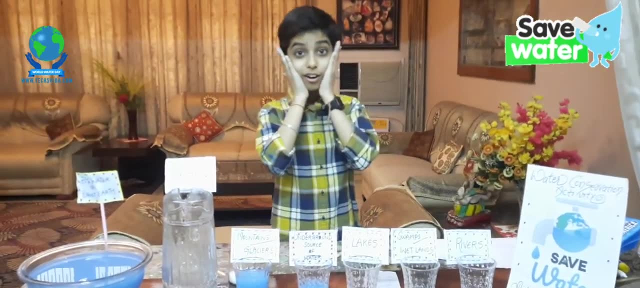 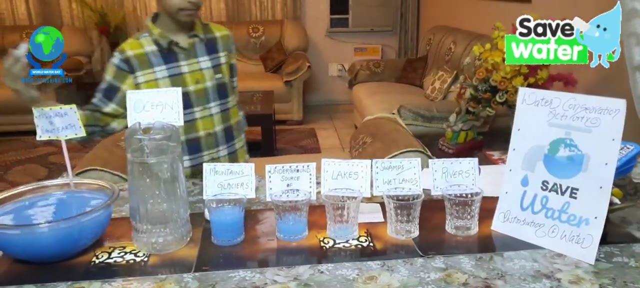 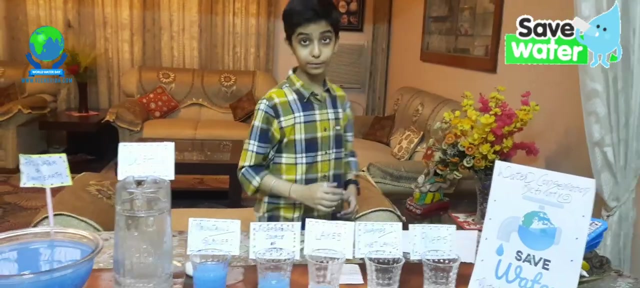 less. how much for oot is in swamps and wetlands? only five drops, literally. can you imagine? only five drops, oh my gosh. now I'm going to put five drops. this is the drop up, and this is five drops. and now it's turn of rivers. there are so. 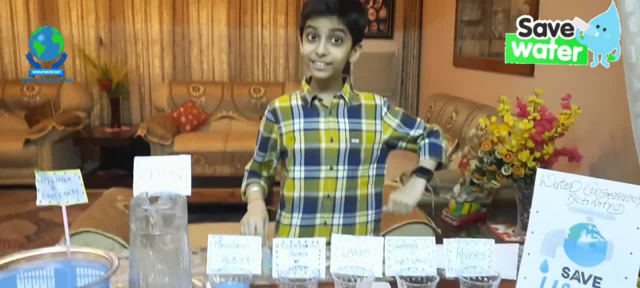 many various swamps and wetlands and I hope you can see there are so many swamps and wetlands and I hope you can see there are so many big rivers in the whole world. can you now guess rivers? amount of water: no, only 0.02. 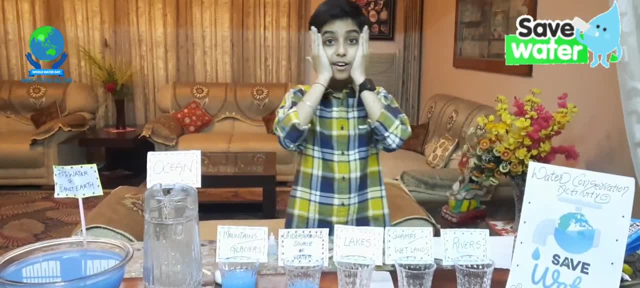 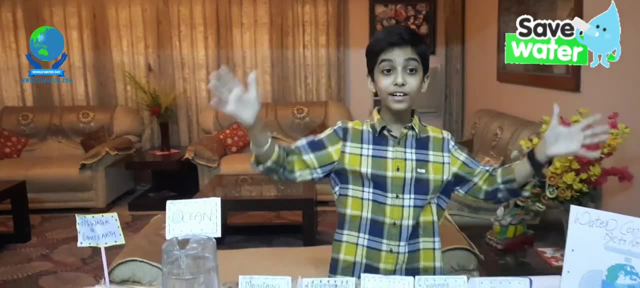 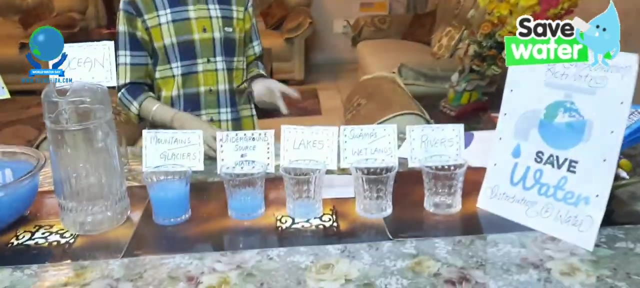 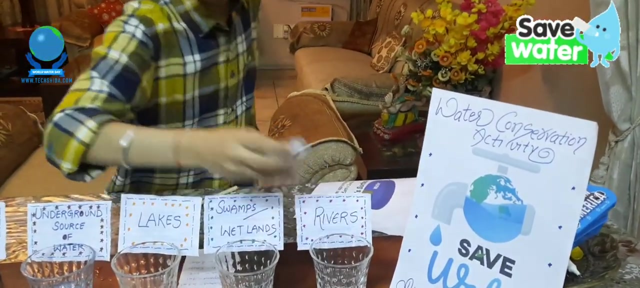 only two drops of water. oh my god, oh my freaking god, only two drops. we have such big rivers in the whole world and only two drops out of this whole water in the planet earth. i cannot believe. but it's true and that's it. only two drops in rivers. i cannot please stay. only rivers have, only two. 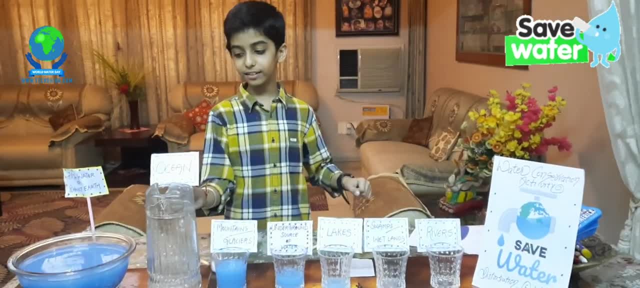 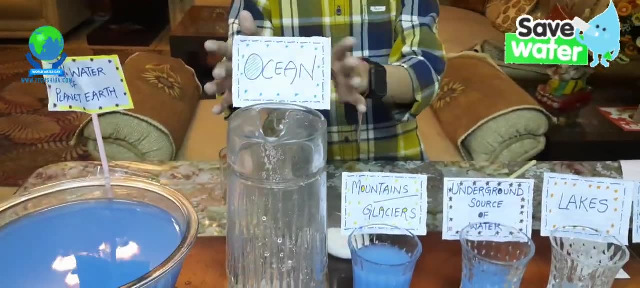 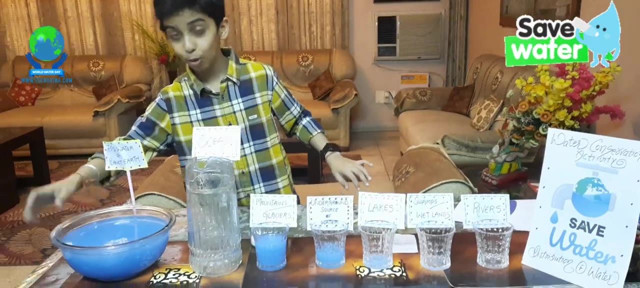 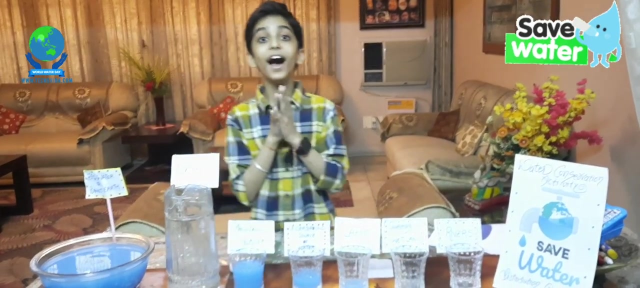 drops of water. and now one is remaining, last one, which have a big container. its name is ocean. and now can you guess how much water oceans have? this whole container water is. now i will put in oceans. the oceans have: 970 ml of water means 97. 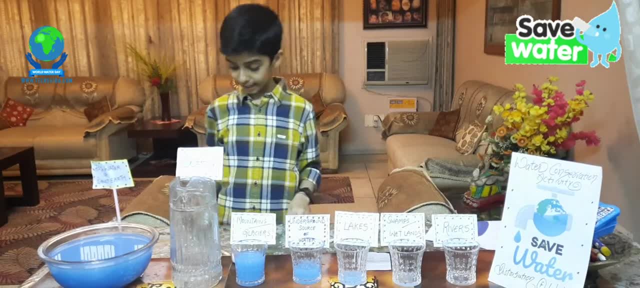 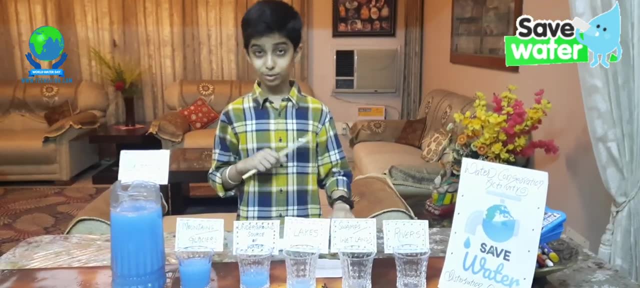 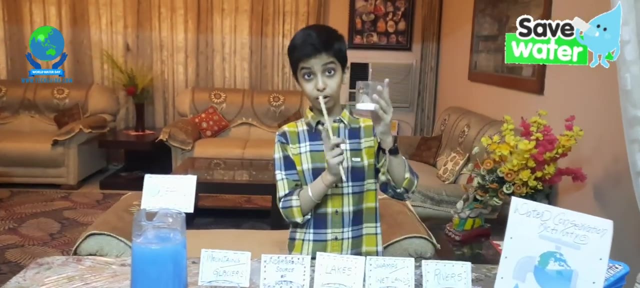 of water on this whole planet earth, and now i am going to put 970 ml of water in oceans. so now you will say, then what's need to say water? no, now here you can see its salt, and now i'm going to make this, mix this salt into this whole ocean water. 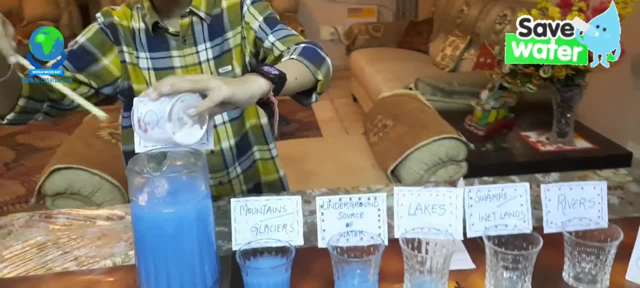 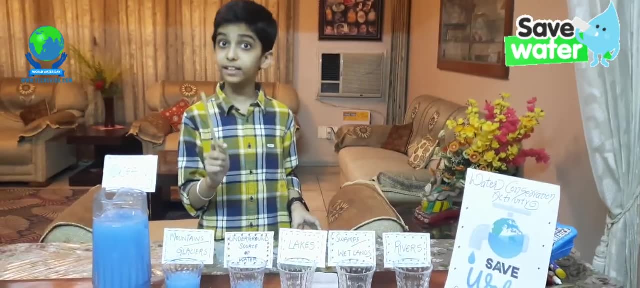 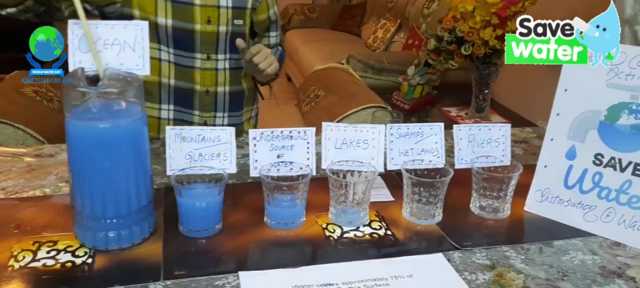 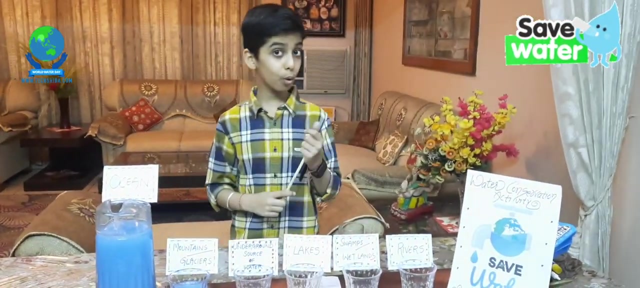 now this ocean what is salty and we cannot drink it. that's why i said been starting that 97 of water is salty and we cannot use it in our in our household works or today. so this is the whole 97 with existing oceans. now you will know that we need save water. so, my dear 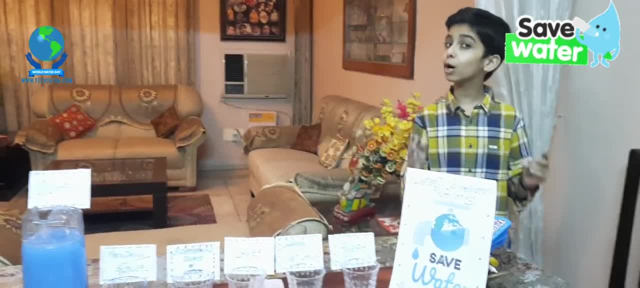 friends, save water, as every drop of water counts. thank you.